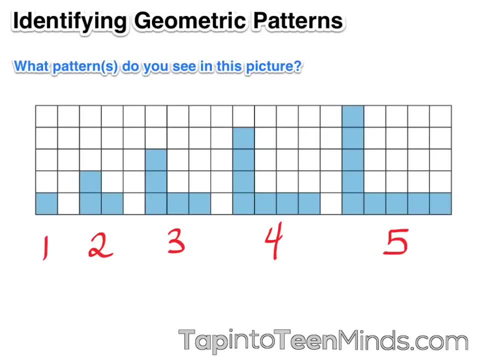 recognize different patterns. One pattern you might notice. if we think about the patterns in terms of their length and width, you'll notice that the first figure has a length of one and a width of one. The same can be said for the second figure, except. 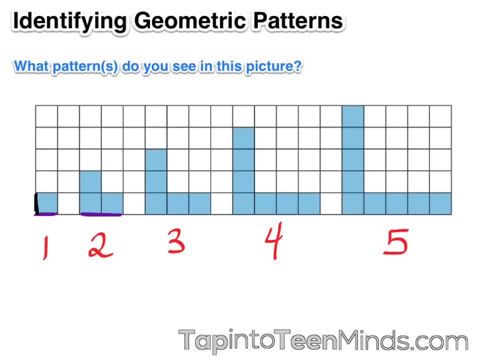 in this case, the second figure has a width of two and a length of two, Or a length of length of 2 and a width of 2.. And you'll notice that this pattern will continue on, going 3 by 3, 4 by 4, and finally 5 by 5.. That's just one example of a pattern that you may. 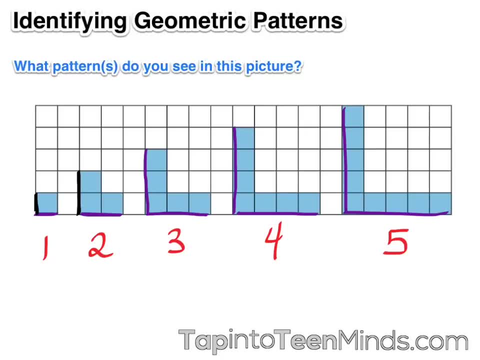 see. Others might notice that if we count the number of squares, there may be a pattern as well. So let's take a look at Figure 1.. Since there's 1 square, we could count a tally above and say there's 1.. In Figure 2, you'll notice there are 3 squares filled in. In Figure. 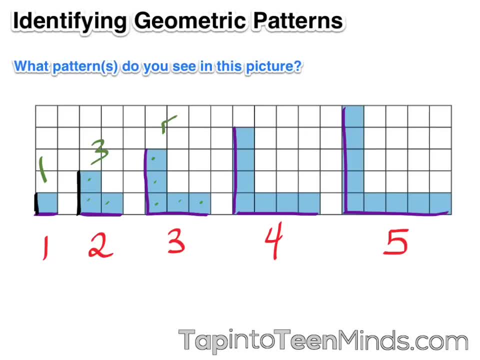 3, 1, 2, 3,, 4, 5.. 5 squares filled in, followed by 7 and 9.. And if you take a moment to think about this, you'll see that each time the number of squares goes up by 2.. So that's another example of 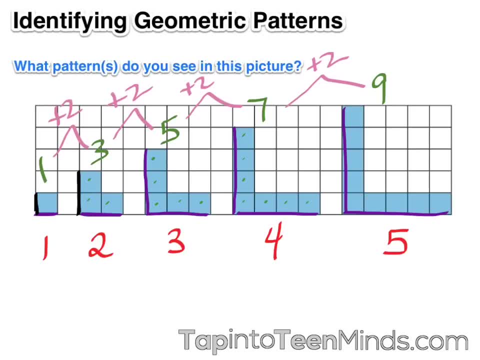 a pattern. One way we can explain our pattern would be through a sentence. An example of a sentence that we can use to describe the second pattern, where we count the number of squares, would be as follows: The sentence I chose to use was: as the figure number increases by 1,. 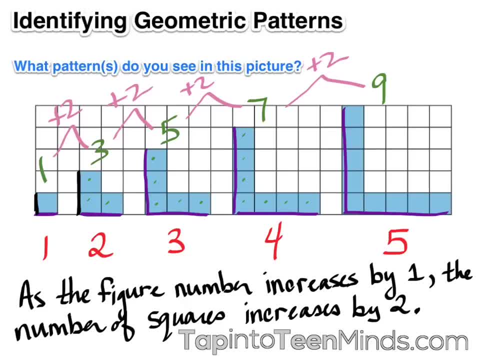 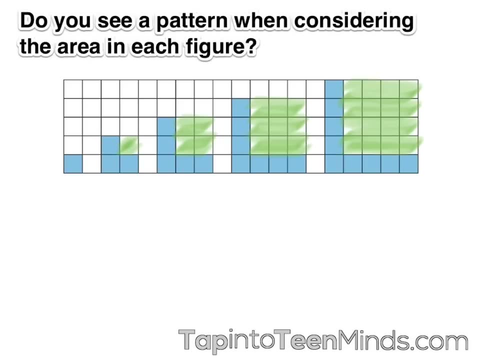 the number of squares increases, The figure number increases by 2.. So you'll see that there is a relationship, and we have described the relationship by first looking at the figure number and then discussing what happens to the total number of squares. In this next case, I've taken the same image, except I'd like you to think about the area. 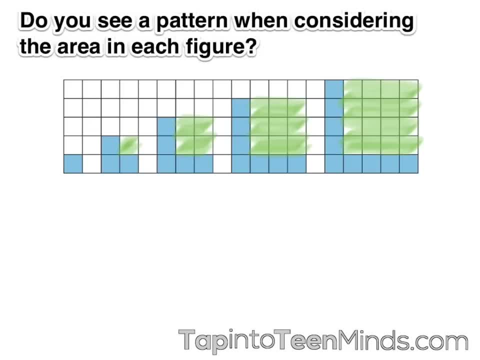 in this particular situation. Take a moment and pause the video to think about the pattern that you may see as the figure number increases by 1.. Now, although there is more than one pattern that you may see, one pattern could be counting the number of boxes total or squares total. Once you've solved that, you can count down. 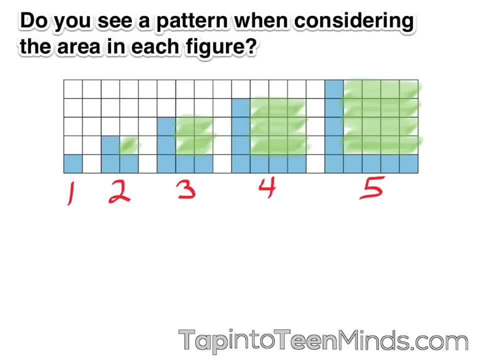 Once again, and in this case let's take a look at the pattern we see here. There's a total of 1, a total of 4, a total of 9, then a total of 16.. You may notice there's a pattern here. 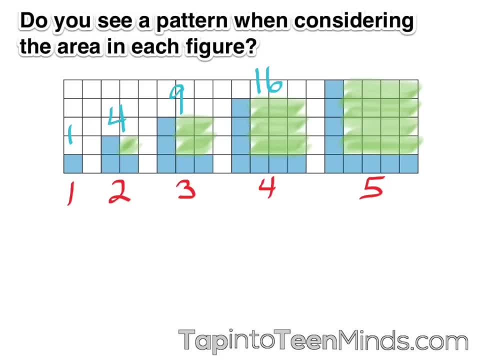 And finally, if we count up all the boxes in the 5th, we have a pattern or a total of 25.. And some people may recognize that 5 squared is 25.. The same could be said about 4 squared, 3 squared, 2 squared and even 1 squared. 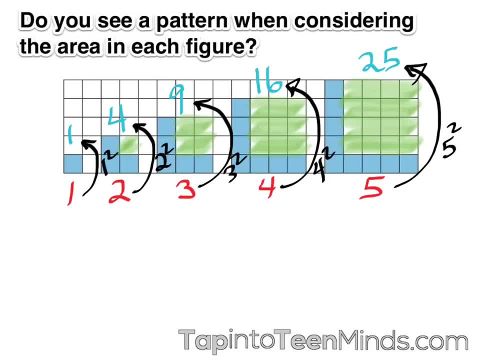 Which explains why we talk about area, how we talk or we speak of area in square units. A sentence to explain the pattern you see might be that, as the figure number goes up by 1, the number of squares is equal to the figure number squared. 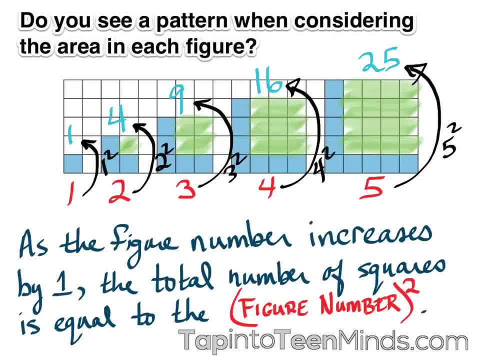 As the figure number increases by 1,, the total number of squares is equal to the figure number squared.